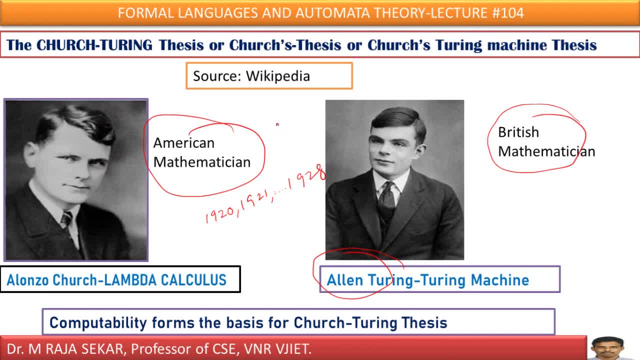 the, the, the Among people, means these. computability is not defined in precise manner. There is no proper definition or I can say there is no proper explanation for a word known as computation or computability. In order to address this problem, in order to explain what is computability, in order to precisely state what is computation, 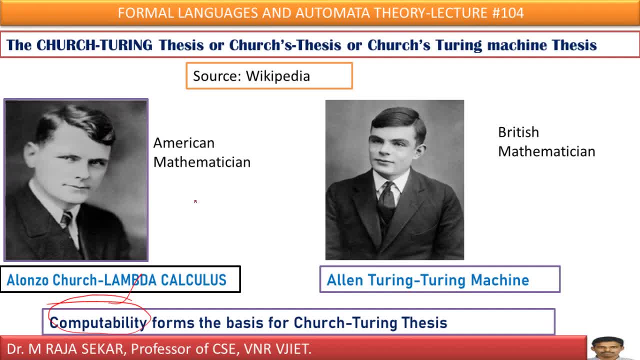 Two mathematicians proposed two different models. First, mathematician Alan J Church, who introduced a mathematical model or machine known as lambda calculus, whereas Alan Turing is introducing a mathematical model or a theoretical model or a Turing machine to explain what is computability or what is computation. 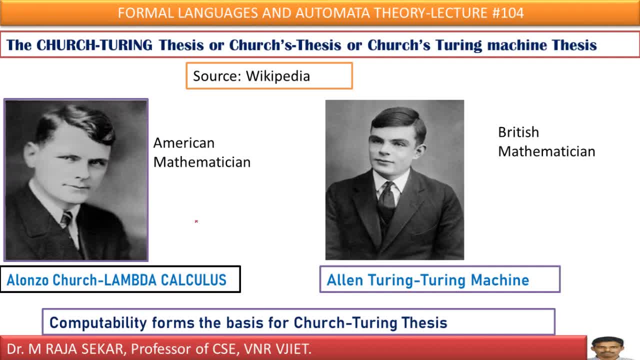 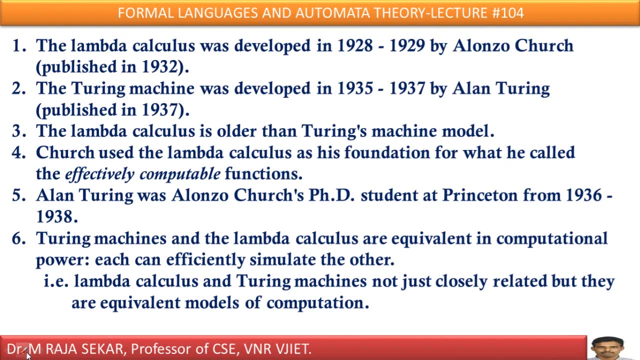 Before discussing this Church-Turing thesis, let me share few words about these two genius mathematicians. As I told you in my previous slide, this lambda calculus is introduced by Alan J Church. The lambda calculus was developed in the year 1928 to 1929 by Alan J Church. 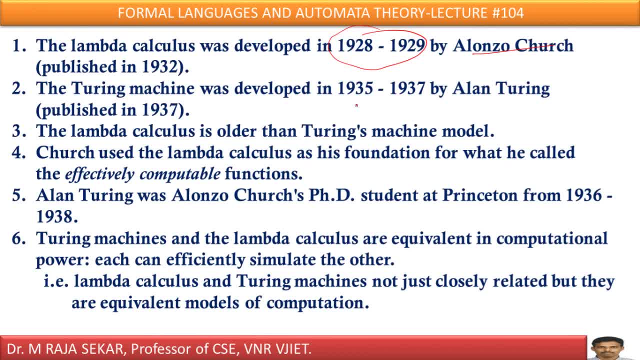 It's published in 1929. It's published in 1929. It's published in 1929. It's published in 1932. The Turing machine was developed in the year 1935, in between 1937.. Just if you observe these two dates, which one is introduced first? lambda calculus is: 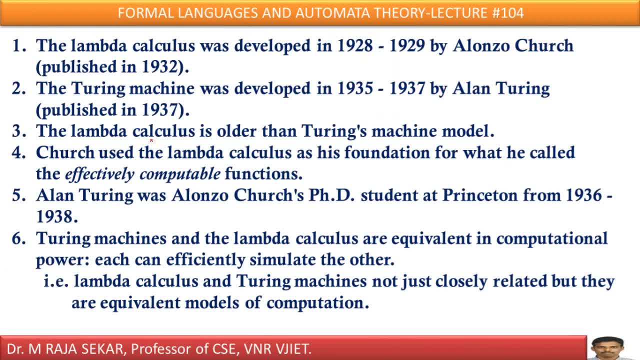 introduced first. Therefore I can say lambda calculus is older than Turing machine model. Church used lambda calculus. I already told in my first slide itself. Church used lambda calculus to explain what is computability and what is computation and what is computable function. 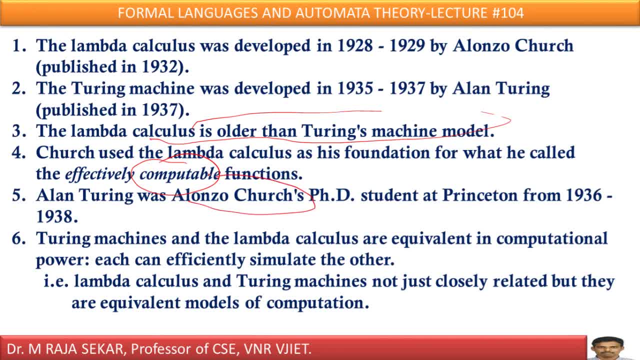 In similar manner, Alan J Church used Turing machine to explain what is computable, what is computable function and what is computation. He used Turing machine. Yes, surprisingly, Alan Turing was Alan J Church's PhD student at Princeton from 1936. 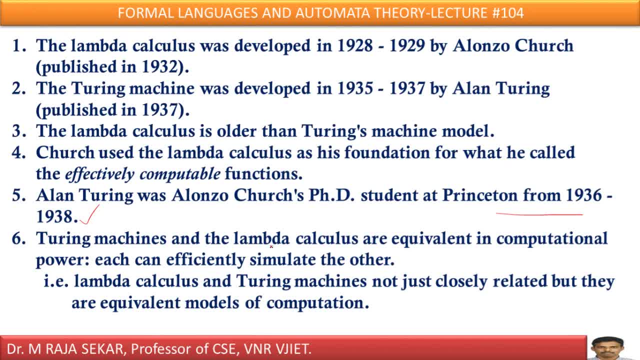 to 1938. Turing machines and lambda calculus are equivalent in computational power Means they are equivalent. The Turing machine expressive power and lambda calculus expressive power is same, That is, Turing machine can simulate lambda calculus machine. Lambda calculus machine can simulate Turing machine model. 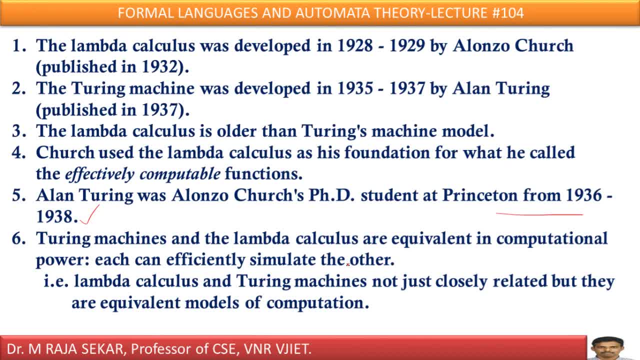 That is, each can effectively simulate the other, That is lambda. calculus and Turing machine machines are not just close, They are closely related, but they are equivalent models of computation. Here, heart of this Church-Turing thesis or Church thesis is computation. 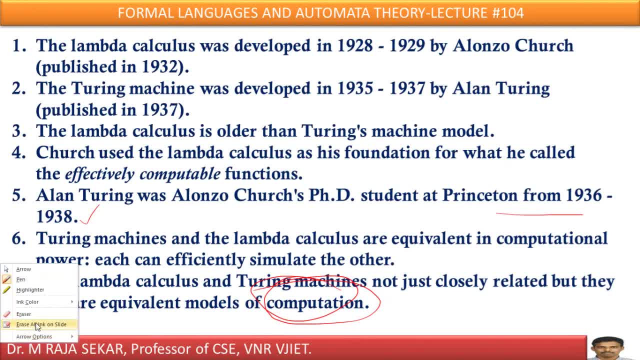 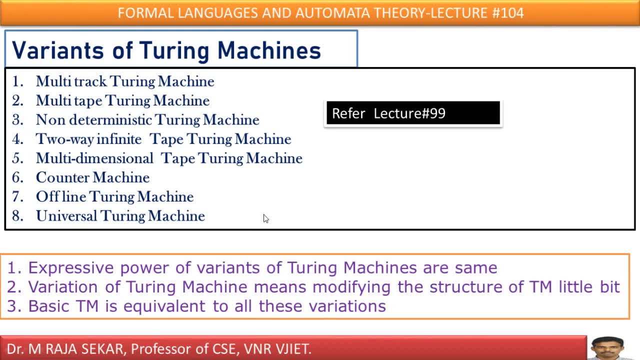 These are the persons, These are the great mathematicians who explained computability or computable function with lambda calculus and Turing machine. Now I can say something about variants of Turing machine in the context of Church-Turing thesis or Church-Turing model. 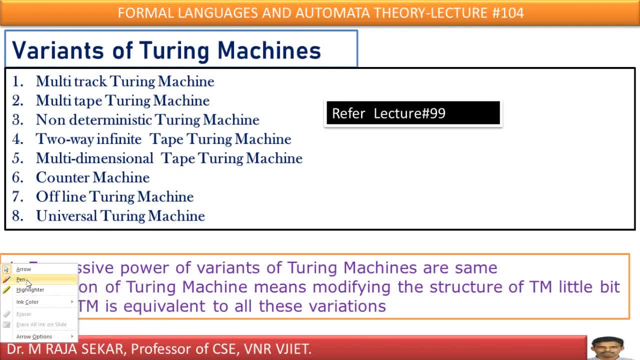 Yes, Let me say in the context of Church-Turing hypothesis, let me say Church-Turing thesis. I already discussed about variants of Turing machines in lecture number 99. I request you to refer once. There may be different variants of Turing machines. 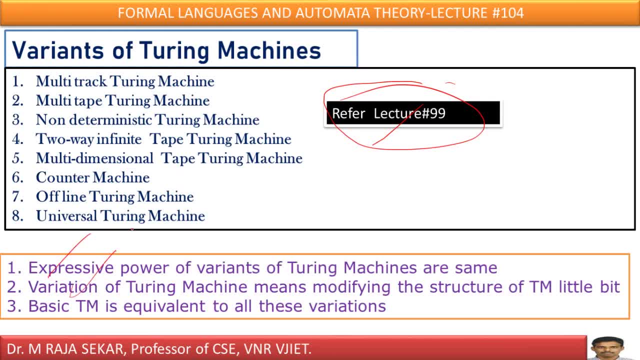 All Turing machines' expressive power is same. All Turing machines' computability power, computation power, I can say computation power. Actually, which one is heart of your Church-Turing thesis? Computability power, Yes, Computability power, Yes. 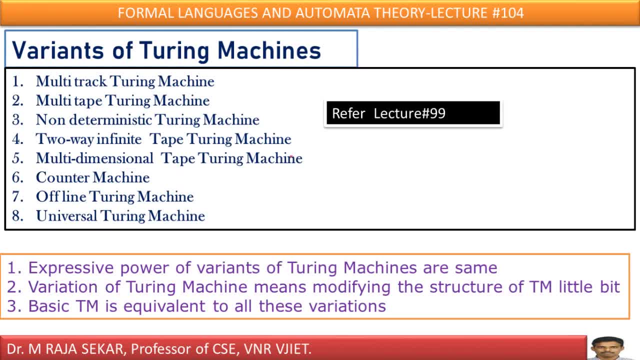 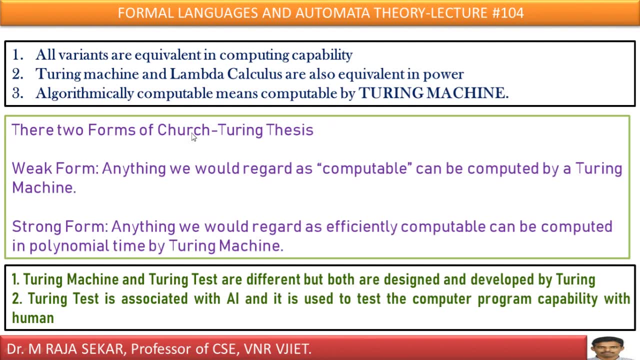 Yes, Computability or computable function or computation, all these variants of Turing machines are equivalent in terms of computability, or in terms of computation, or in terms of computability. Yes, Yes, That's what it says. Again, the same thing I am repeating. 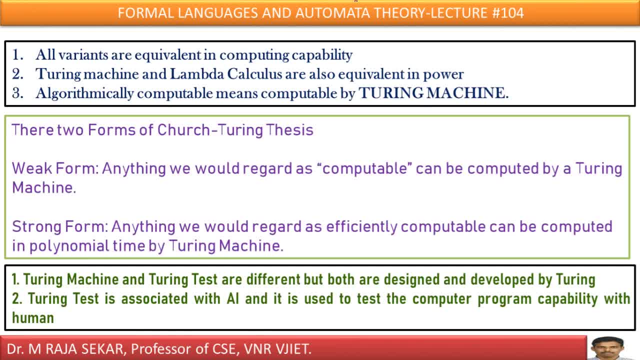 Of course it's not harm in repeating good things again and again: All variants, What it says. All variants are equivalent in computing computation. Yes, Yes, All variants are equivalent in computing computation. All variants are what. All variants of Turing machine are equivalent in computing capability. 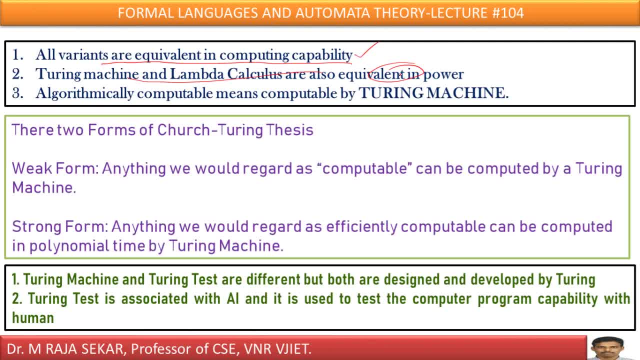 Turing machine and lambda calculus are also equivalent. I already stated this one. Of course it's a good thing. Let me repeat it again. Algorithmically, I can say this: third point is very, very important. This I can say: this is Church-Turing thesis. 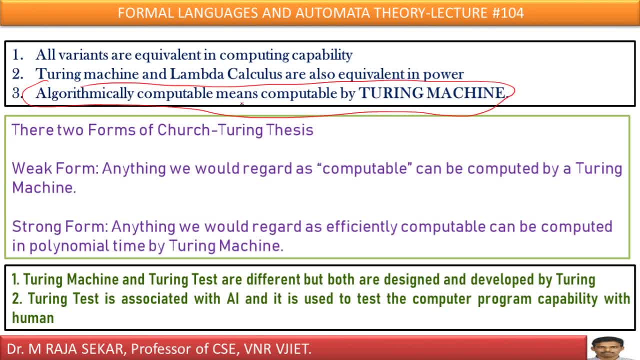 Yes What it says. Algorithmically computable means if you are able to compute with algorithm means certainly it is computable by Turing machine. Algorithmically computable means you are able to compute with Turing machine machine. algorithmically computable means computable by turing machine. if there is something which can 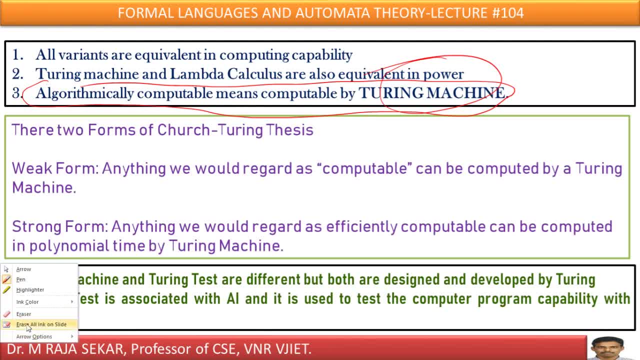 be computed with. algorithm means that can be computable by your famous turing machine. there are two forms of church turing thesis. first form is weak form. second form is strong form. just compare these two forms. what it says, anything we would regard as computable. that's what i am. 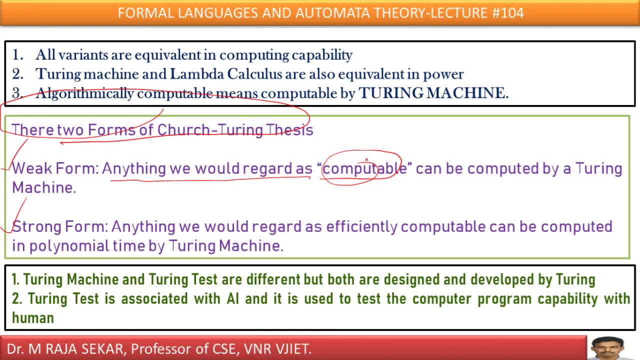 repeatedly saying computation or computability is a core concept, is a heart of church turing thesis. yes, anything we would regard as computable can be, can be computed by turing machine means if something is computable that can be computed by turing machine, that is. that is, i can say. 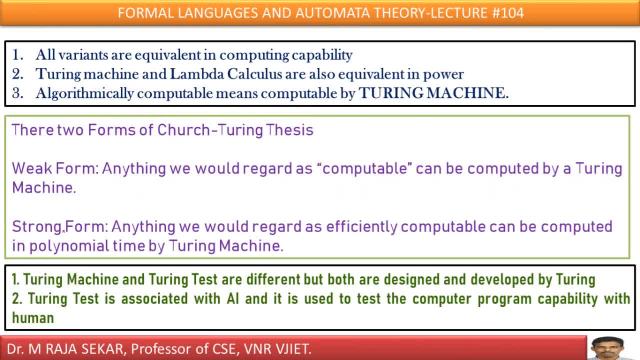 that is weak form of church turing thesis. then what is strong form of church turing thesis? just compare: anything we would regard as, just see, anything we could regard as here. Here we have computability Instead of computability. he is saying efficiently computable. Just he is adding efficient word Can be computed, Just see, can be computed by a Turing machine. Can be computed by a Turing machine, Just see, by a Turing machine. 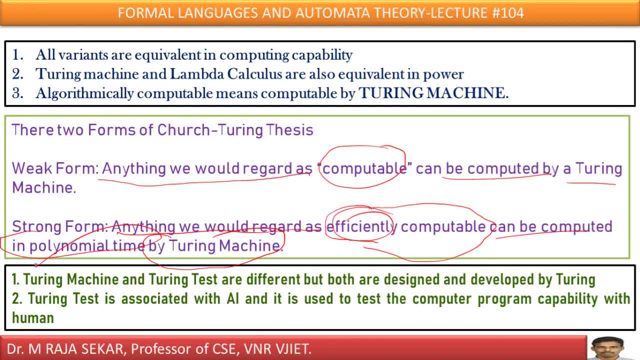 But he is giving time, Polynomial time. He means in strong form. He is saying time complexity and that computation is also efficient. These are two different forms of chess Turing thesis. In the case of strong form, he is precisely saying about time complexity. He is pressing on computability. That's what he is saying: Efficiently computability. 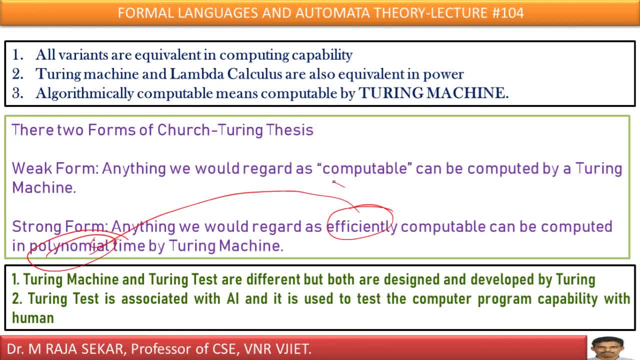 Polynomial time. Because of these two words, this becomes strong form of chess. Turing thesis: Turing machine and Turing test are different, But yes, there are two concepts you might have heard: Turing machine and Turing test. They are different, But similarity between them is both are designed by our famous Alan Turing.